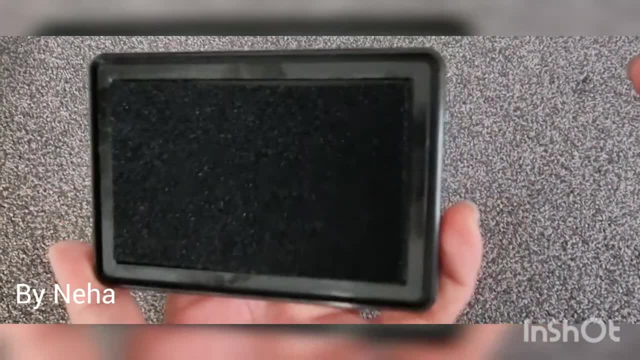 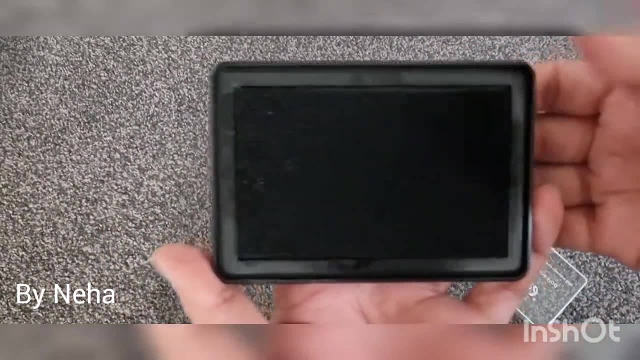 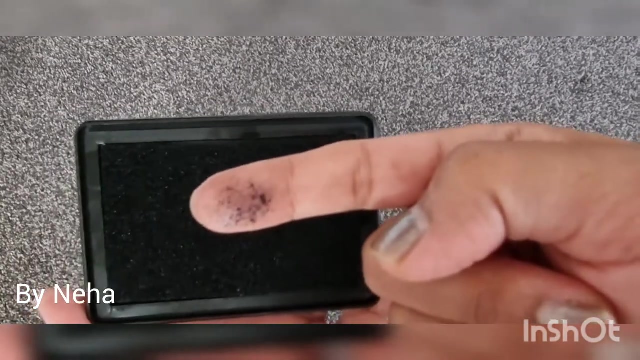 especially for the hands. as the ink is not non-toxic for baby, You can still use them for baby's feet. if you do not find any option, Check the ink with your finger and wipe it off with baby wipes to make sure how easy it is to wipe off from your baby's hands. 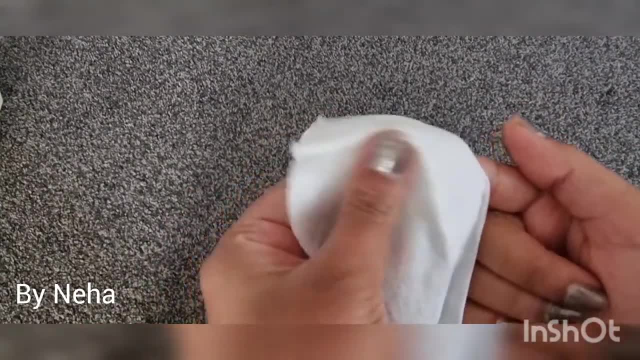 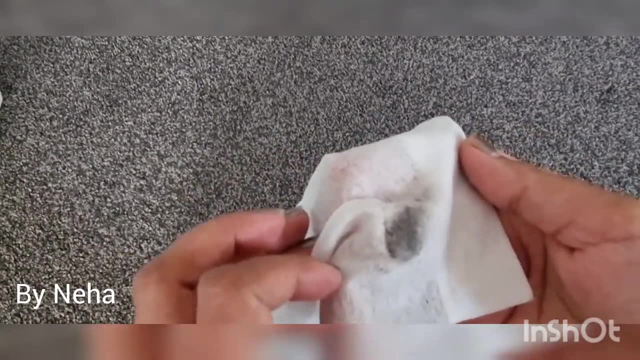 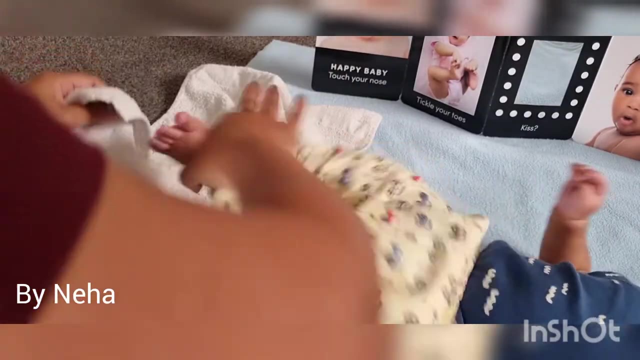 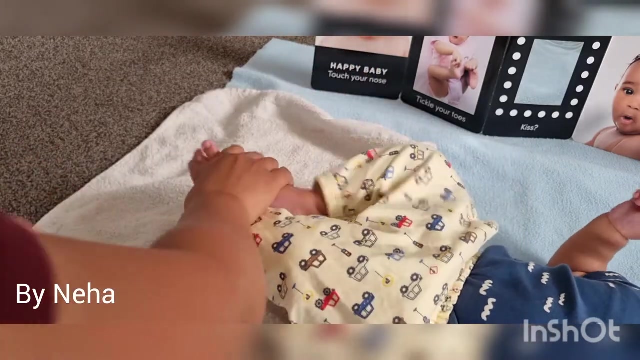 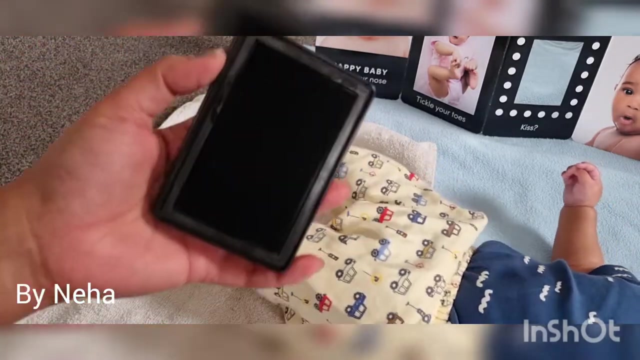 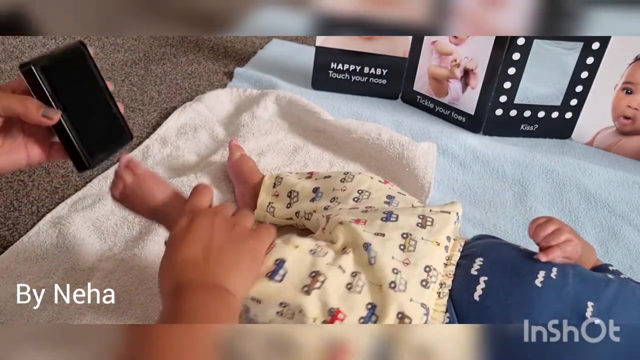 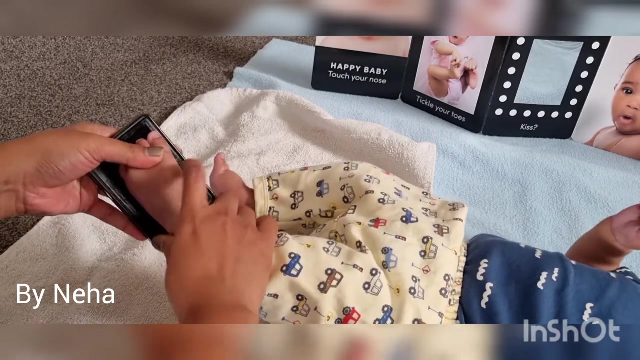 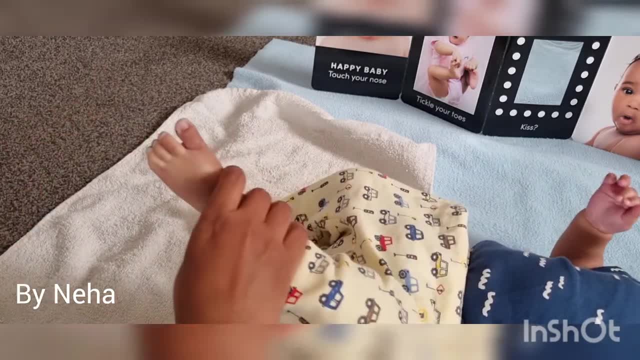 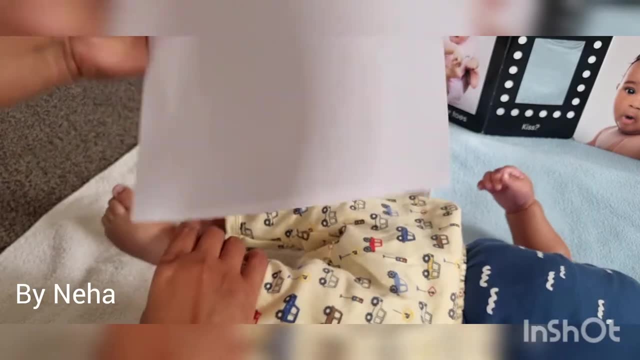 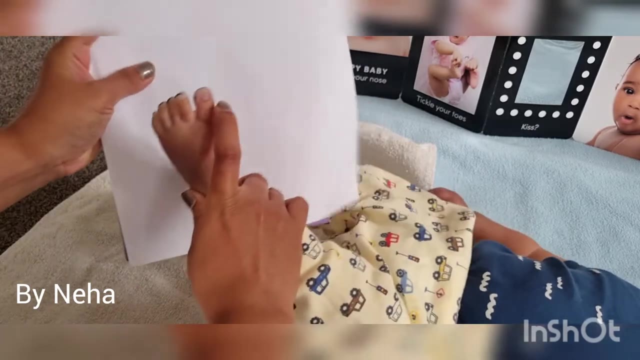 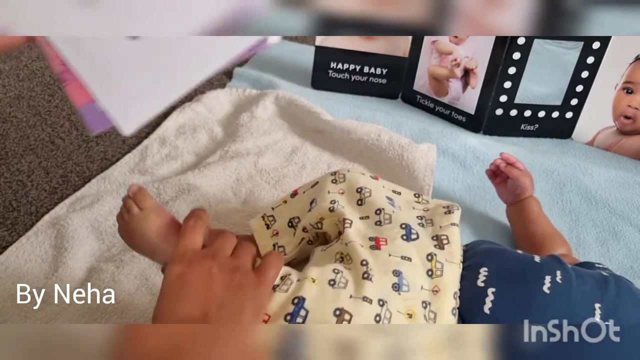 I know it's really difficult. Now take the plain paper attached to an exam pad or a register, as I have taken behind for a foam support. Gently press baby's foot over the paper, either in the air while the baby is sleeping on his back, or you can take someone's help to hold baby in a standing. 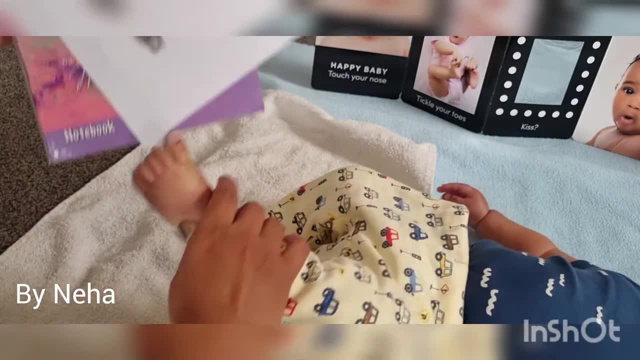 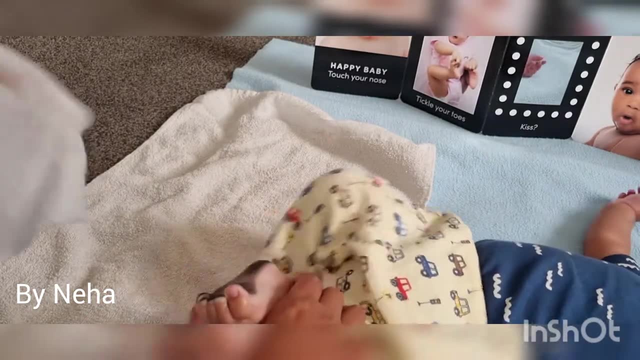 position over the paper. Repeat the stamps of feet and repeat the steps. You might feel full of confidence and can also believe that you are going to get the marker. Now take the stamp pad and flip it over so the baby can come out of the pad. 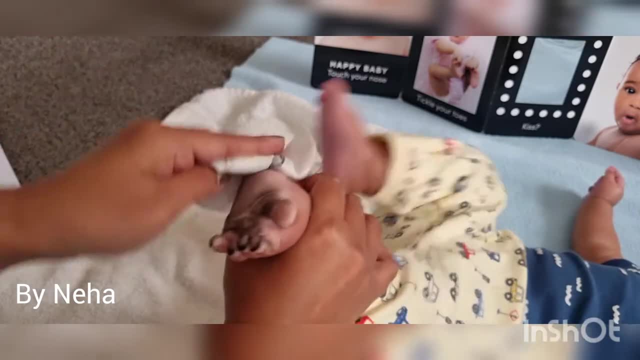 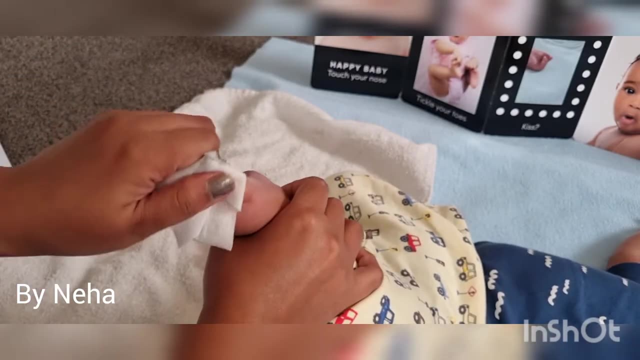 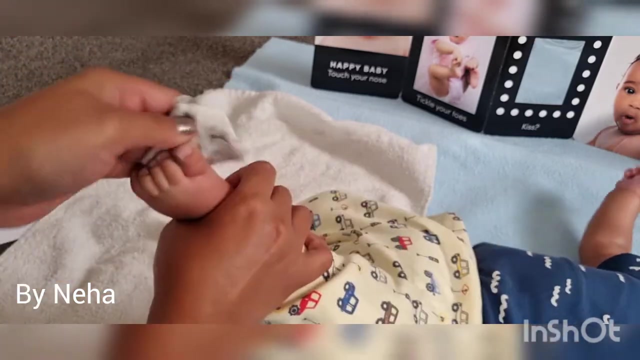 White of the ink with the baby wipes. White of the ink with the baby wipes. Then take the stamp pad and flip it over. Then take the stamp pad and flip it over so the baby can come out of the pad. Now open the stamp pad.